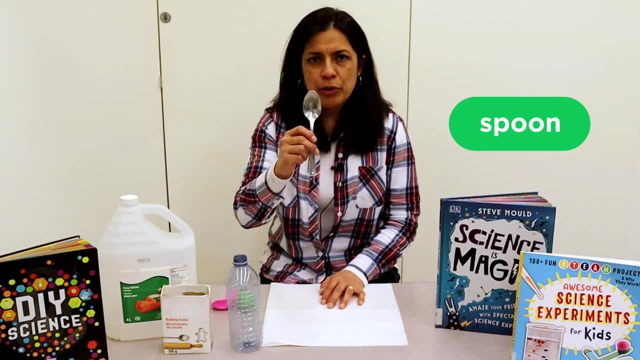 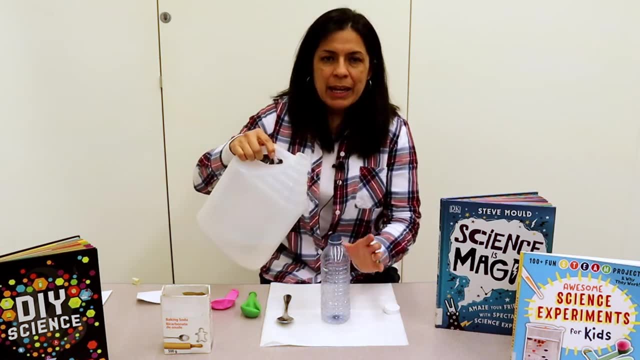 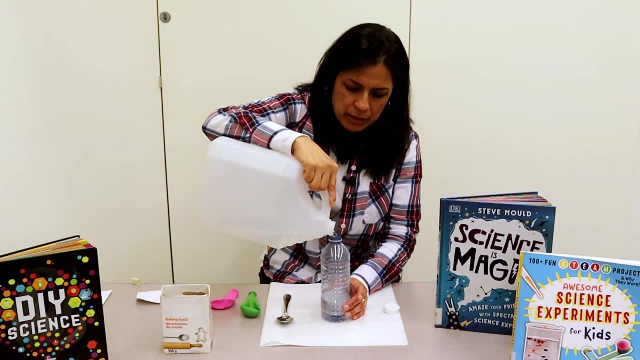 some baking soda, an empty plastic bottle of water, a spoon and a balloon. Let's start by pouring our vinegar into the bottle. We need about half cup of vinegar, and you can always ask your mom or your dad to help you with this step. Perfect, Let's leave the bottle aside Now. 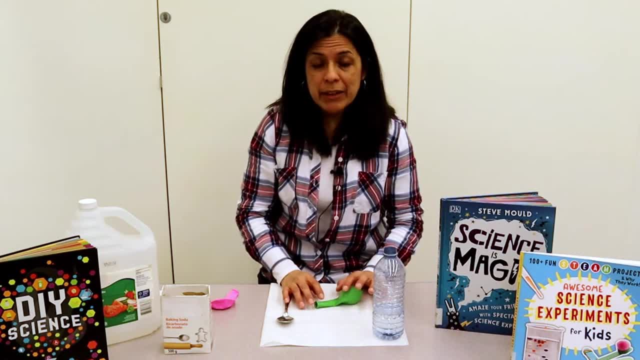 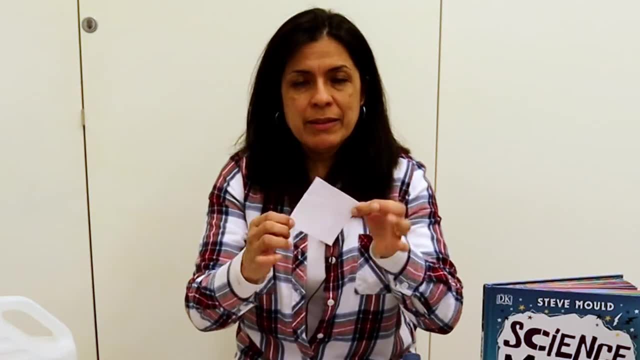 let's grab our balloon, And this step is easier if you have a funnel handy. I don't have one, so I'm going to make one. You need a small piece of paper like this, a simple piece of paper, and I'm going to put my finger in one of the corners. 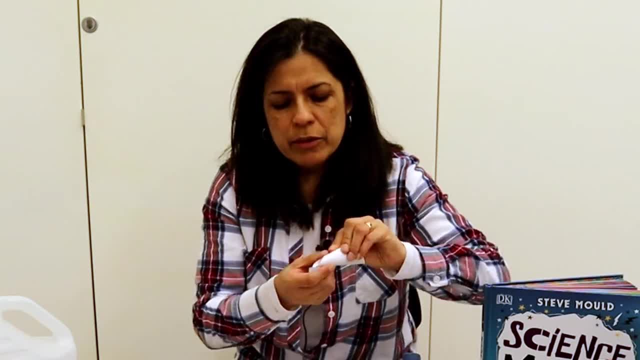 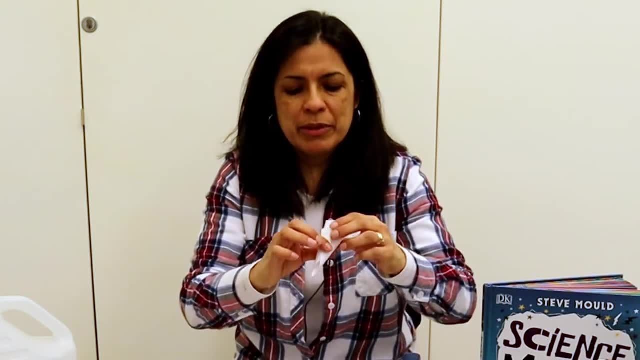 and just wrap it around my finger like this: Make sure that we leave a small hole at the bottom, And then you can just use a small piece of tape just to attach it. We have our funnel. So with the help of the funnel, 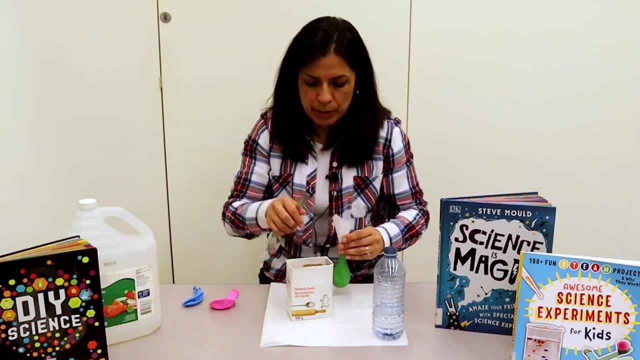 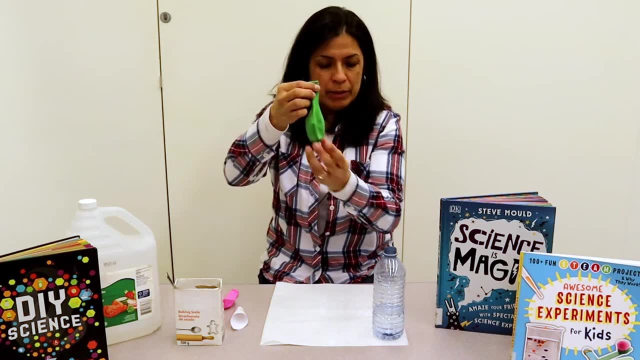 we're going to put it inside of the balloon and we are going to scoop two tablespoons of baking soda. Make sure that everything goes in. So we have the baking soda in the balloon, we have the vinegar in the bottle. So now let's attach the balloon to the bottle. 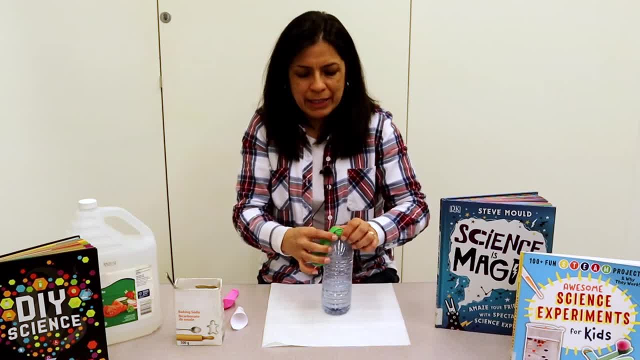 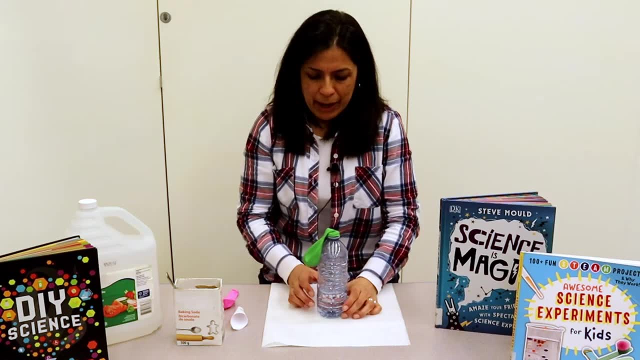 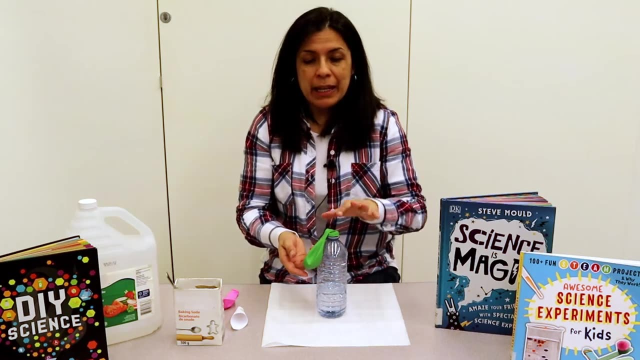 making sure that it's really tight. Also, don't let this baking soda go into the vinegar. okay, Like this. So now let's count to three And we are going to lift the balloon and allow the baking soda to go into the bottle. 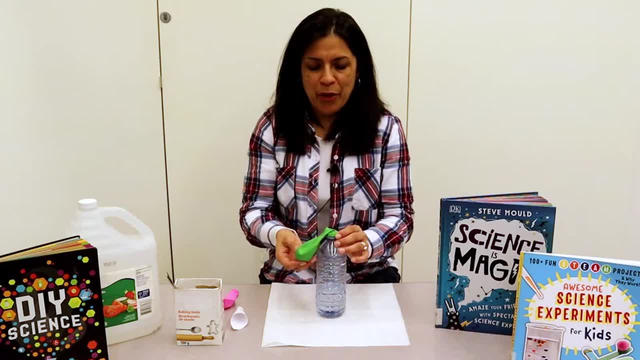 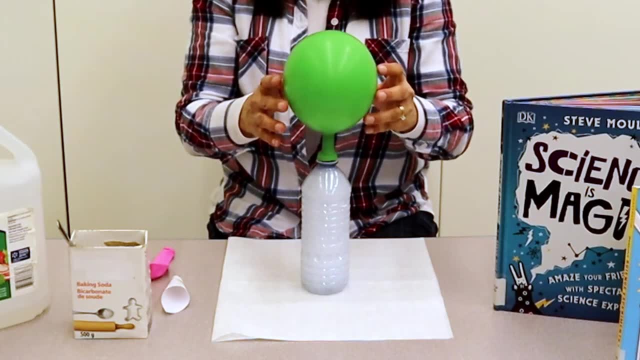 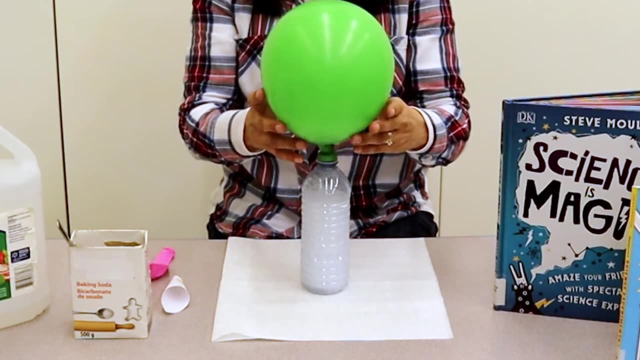 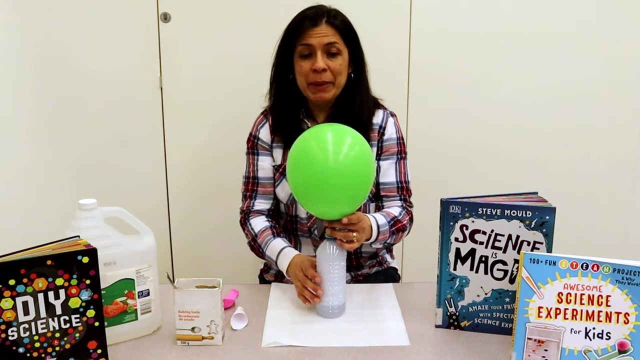 Ready. One, two, three, Whoops, Wow. So the reaction is inflating our balloon. But why does this happen? When we mix a base- that in this case is the baking soda- with an acid that is the vinegar.